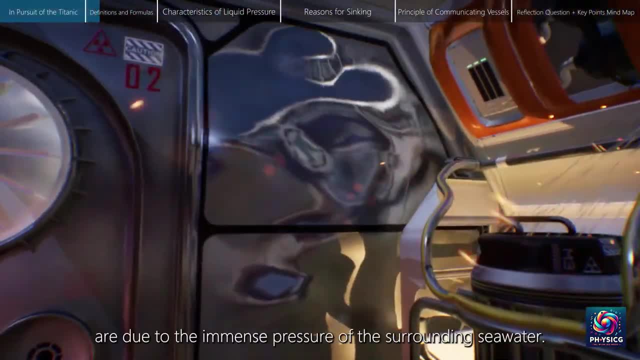 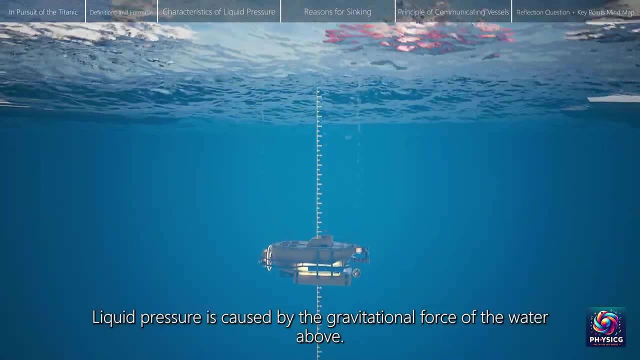 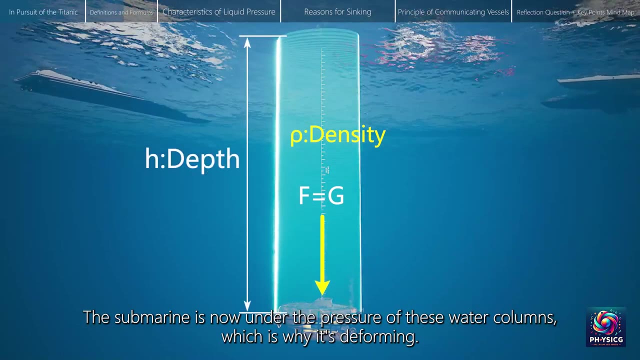 structures to be destroyed. These conditions are due to the immense pressure of the surrounding seawater. Liquid pressure is caused by the gravitational force of the water above. The submarine is now under the pressure of these water columns, which is why it's deforming. 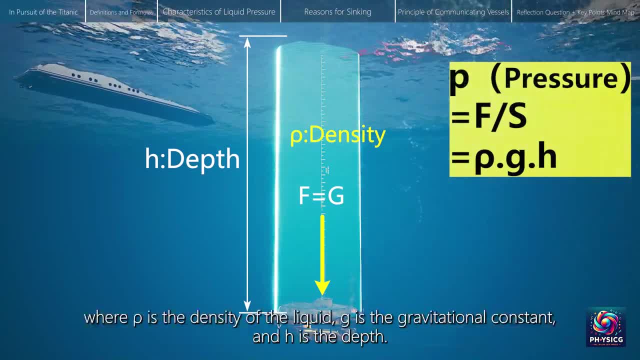 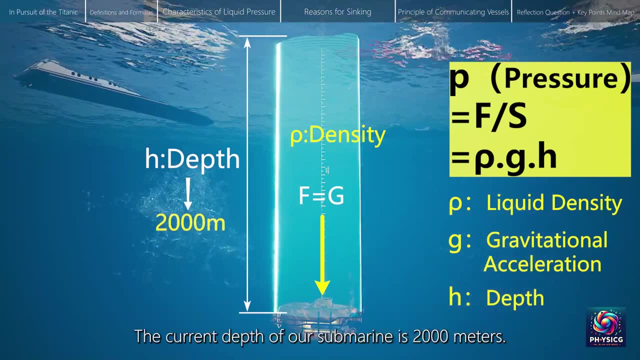 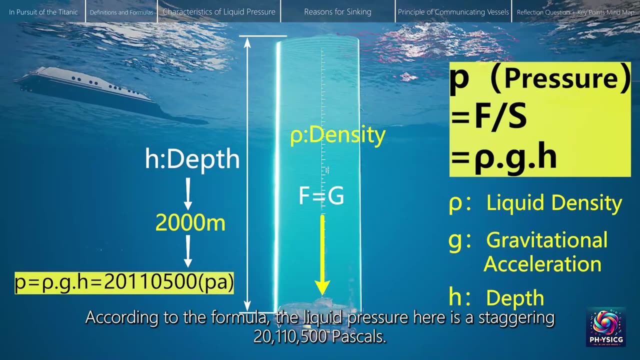 According to the pressure formula, P equals rho, g, h, where rho is the density of the liquid, g is the gravitational constant and h is the depth. The current depth of our submarine is 2,000 meters. According to the formula, the liquid pressure here is a staggering 20,110,500 pascals. 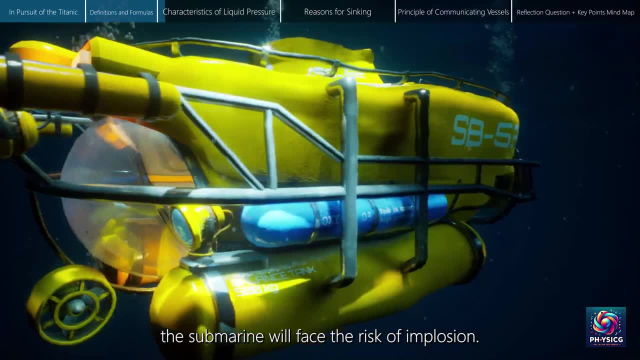 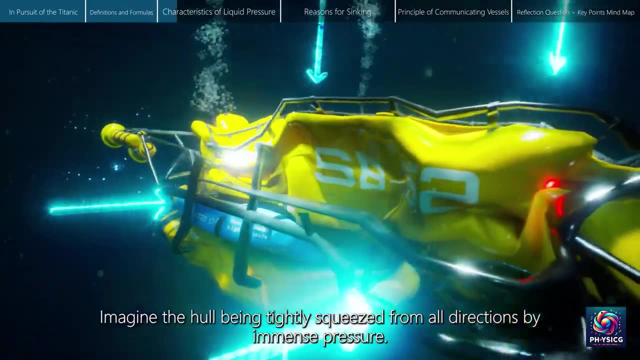 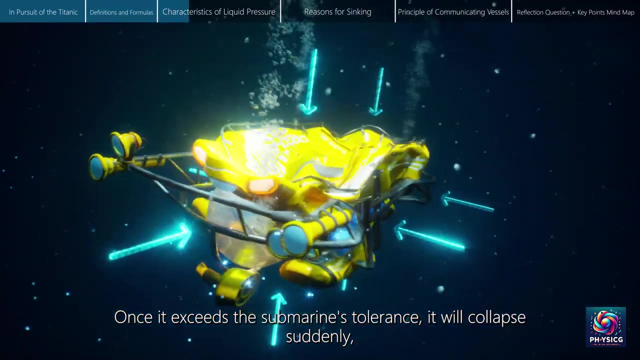 If we cannot repair this damage quickly, the submarine will face the risk of implosion. This is because the pressure of the seawater is applied equally on the hull. Imagine the hull being tightly squeezed from all directions by immense pressure. Once it exceeds the submarine's tolerance, it will collapse suddenly, causing the hard metal to rupture instantly. 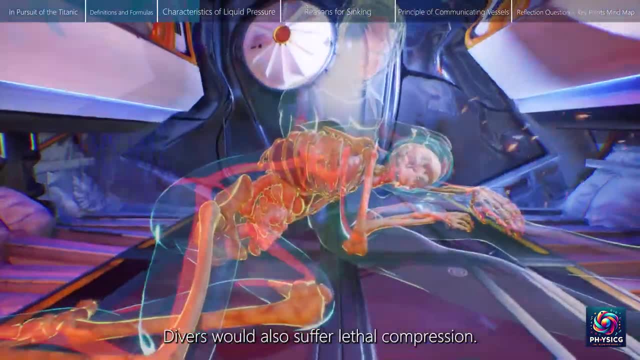 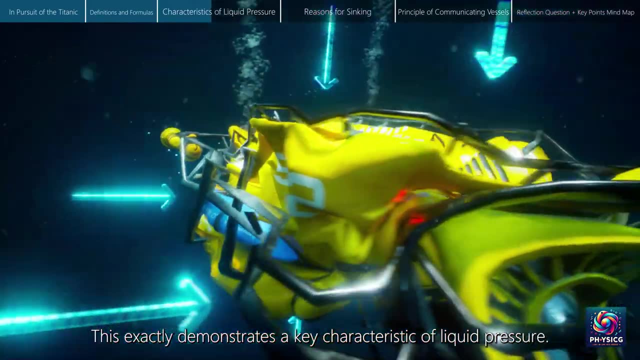 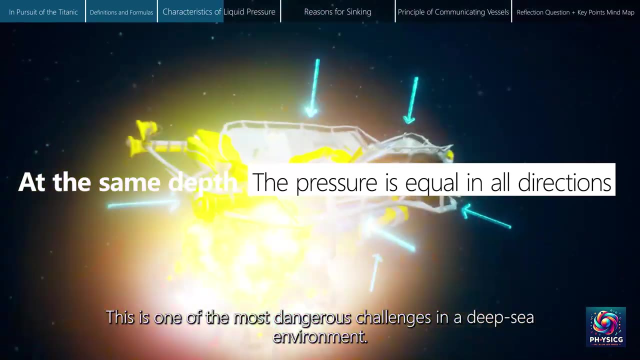 like a tin can being crushed in the deep sea, Divers would also suffer lethal compression. This exactly demonstrates a key characteristic of liquid pressure. Inside a liquid at the same depth, pressure is applied equally in all directions. This is one of the most dangerous challenges in a deep sea environment. 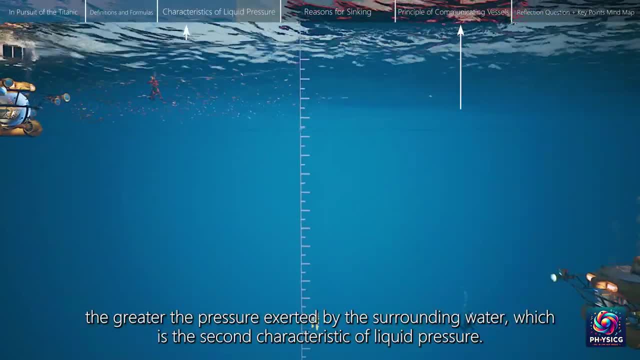 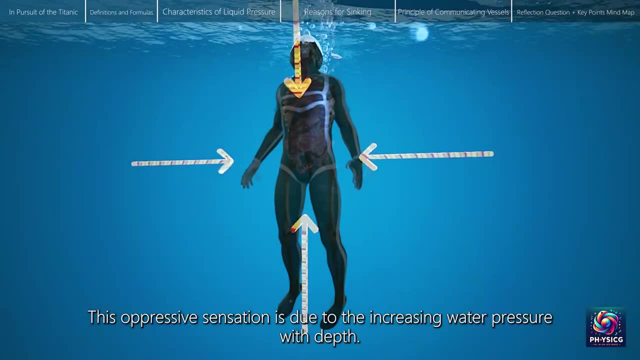 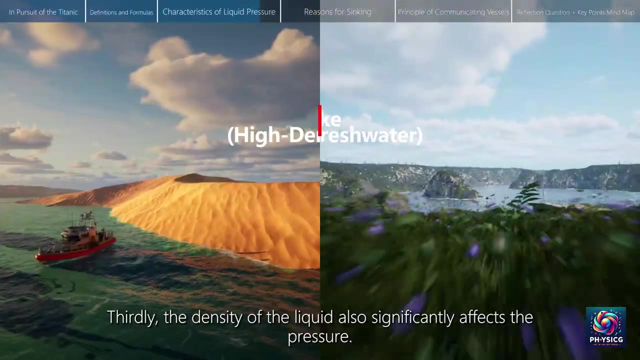 Secondly, as we see, the deeper the depth, the greater the pressure exerted by the surrounding water, which is the second characteristic of liquid pressure. However, this oppressive sensation is due to the increasing water pressure with depth. Thirdly, the density of the liquid also significantly affects the pressure. 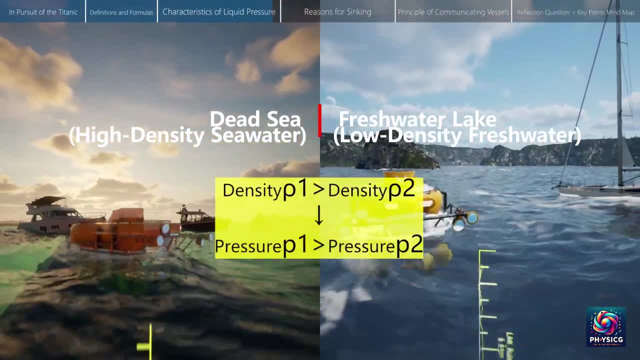 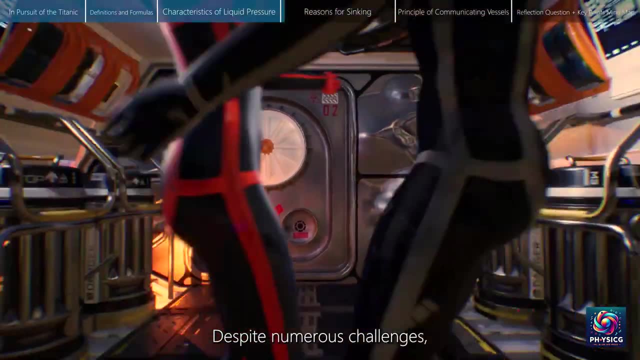 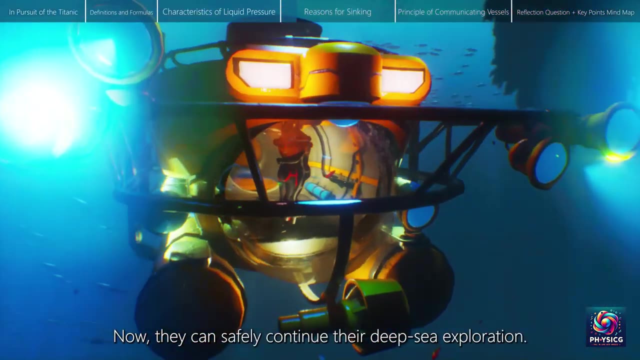 At the same depth, such as in this Salter seawater. the greater density means the liquid exerts more pressure. Despite numerous challenges, this pair of scientists still manages to overcome difficulties and repair the submarine in time. Now they can safely continue their deep-sea exploration. 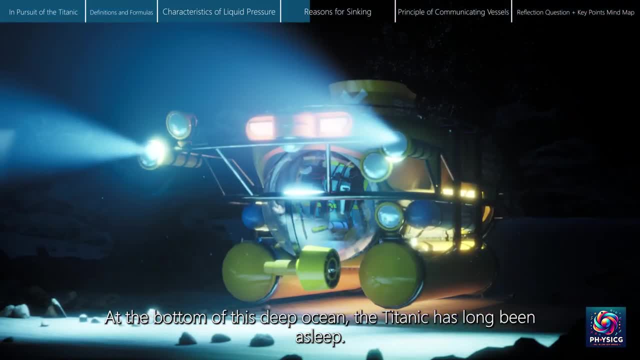 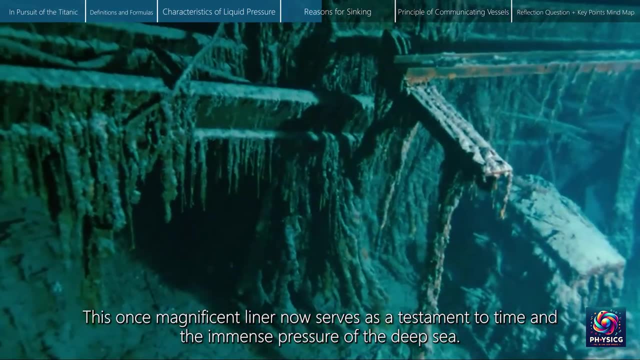 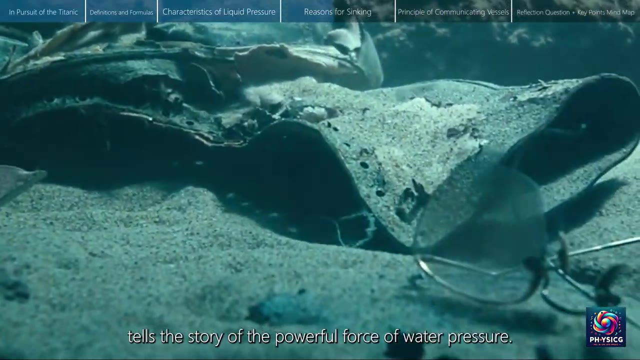 At the bottom of this deep ocean, the Titanic has long been asleep. This once magnificent liner now serves as a testament to time and the immense pressure of the deep sea. Every twisted inch of metal, every shattered piece of glass tells the story of the powerful force of water pressure. 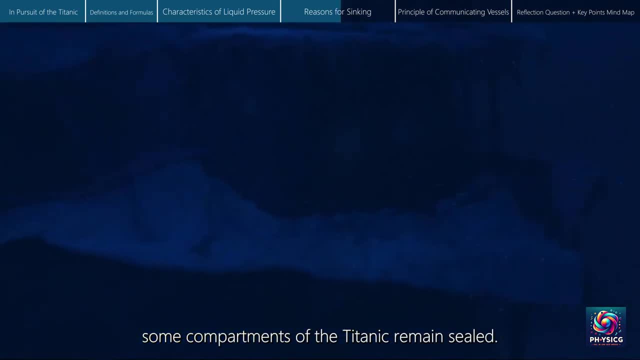 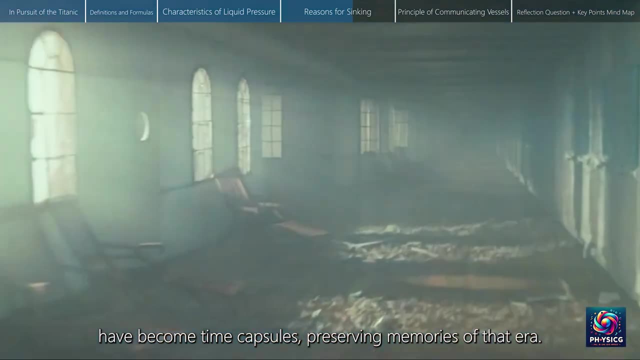 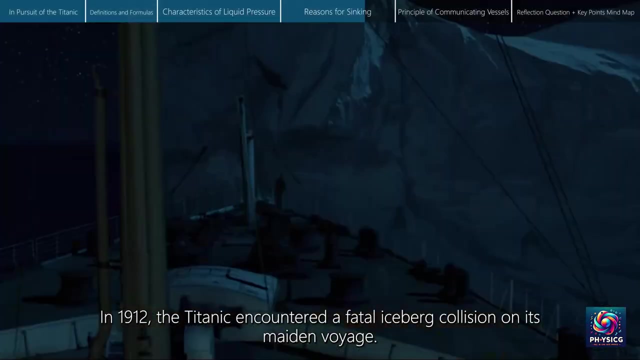 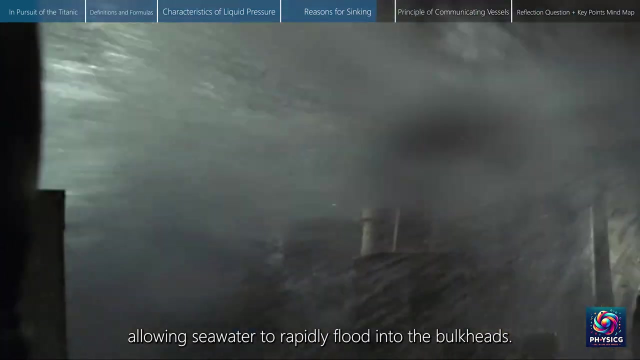 Even under such extreme conditions, some compartments of the Titanic remain sealed Under the pressure. these compartments have become time capsules preserving memories of that era. In 1912, the Titanic encountered a fatal iceberg collision on its maiden voyage. The collision caused damage to the hull, allowing seawater to rapidly flood into the bulkheads. 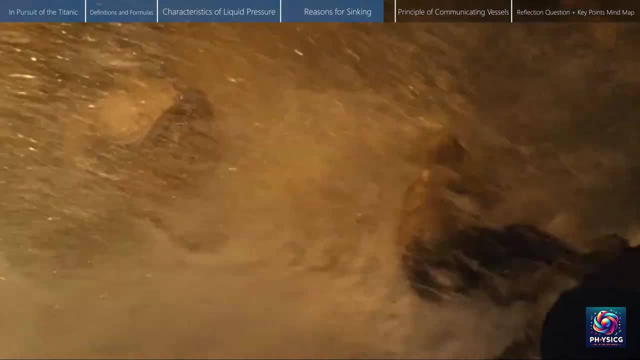 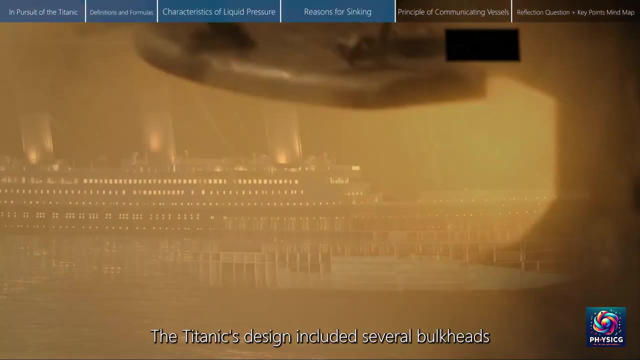 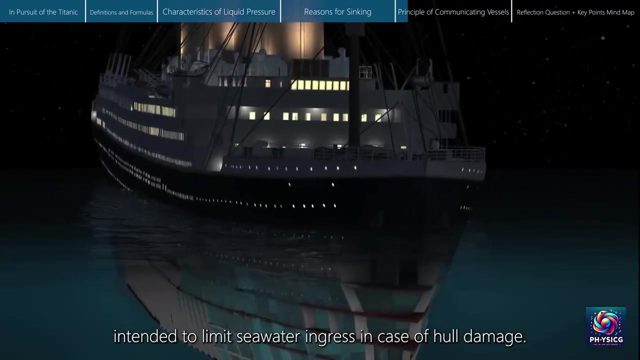 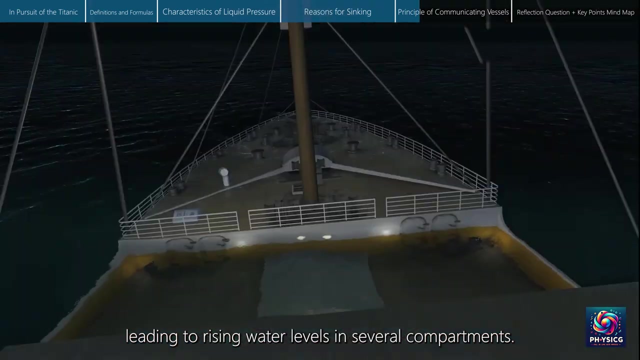 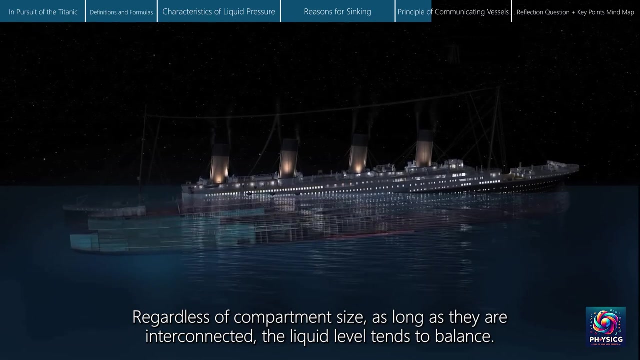 The Titanic's design included several bulkheads intended to limit seawater ingress in case of hull damage. However, the damage compromised multiple bulkheads, leading to rising water levels in several compartments. This is the principle of the communicator: Regardless of compartment size, as long as they are interconnected, the liquid level tends to balance. 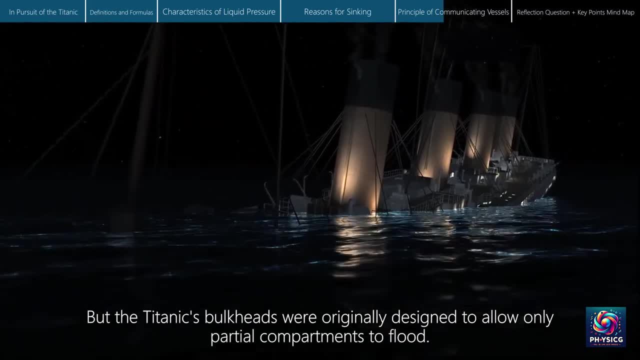 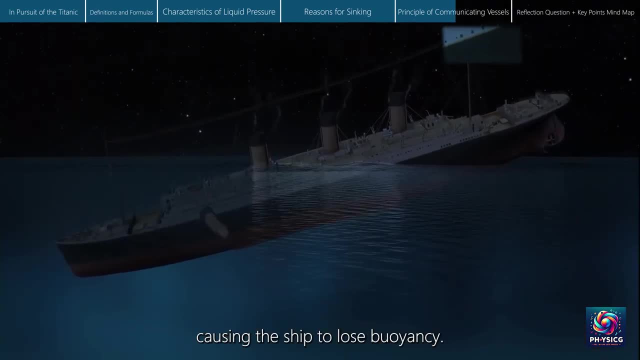 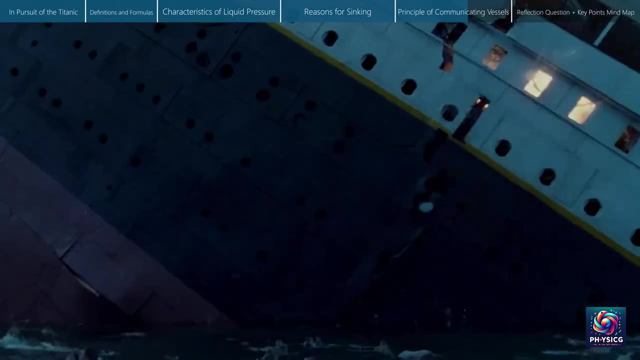 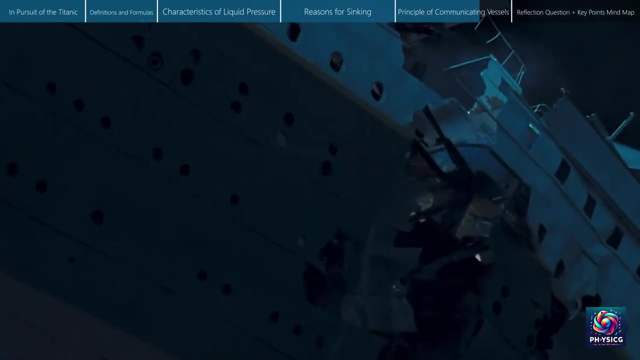 But the Titanic's bulkheads were originally designed to allow only partial compartments to flood. Unfortunately, the extent of the damage was too great, causing the ship to lose buoyancy. The Titanic now features a pieces of the Titanic in the pulse of its containing Beachwater. 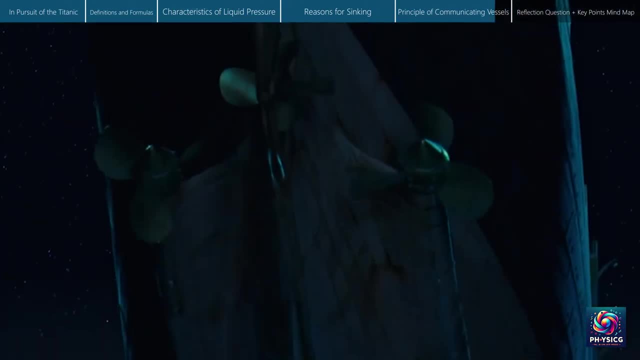 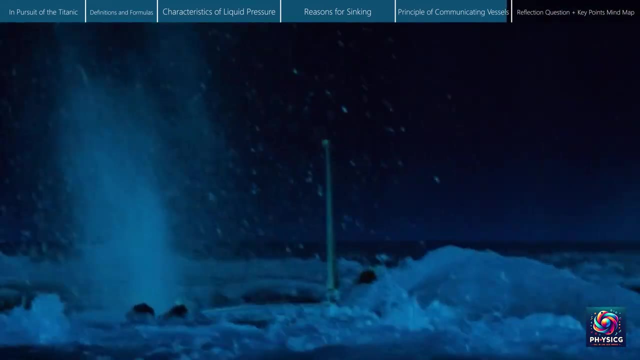 The rail at the end of the Titanic has come off and is running up and down to the surface. All of the ship's bulkheads had been reduced to the ground, leaving one of the hulls damaged by the crash. As a result, a fire broke out and a man was shot and killed. 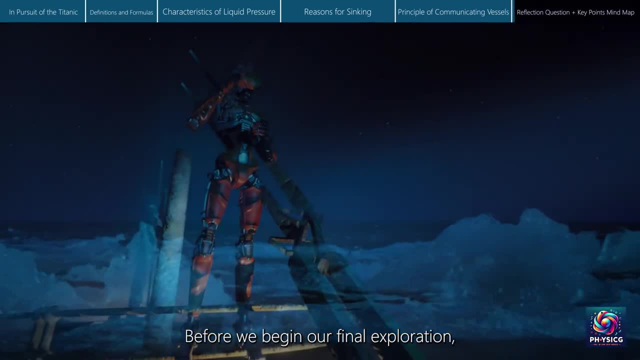 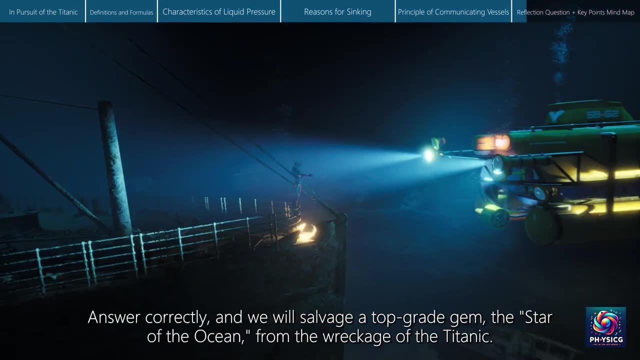 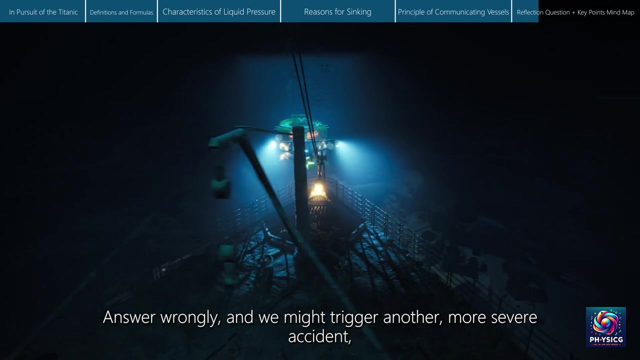 But before we begin our final exploration, there's a crucial question you need to answer. This question concerns our fate. Answer correctly and we will salvage a total wreck of the Titanic top grade gem, the star of the ocean, from the wreckage of the titanic. answer wrongly and we. 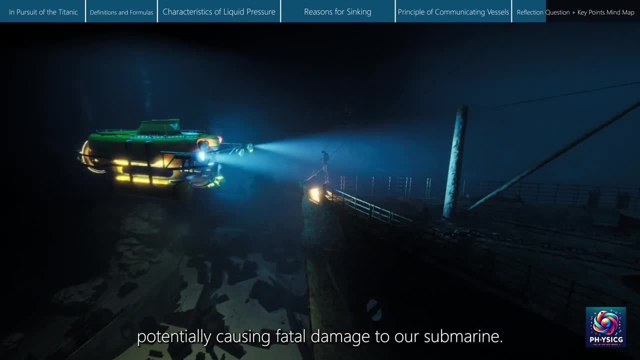 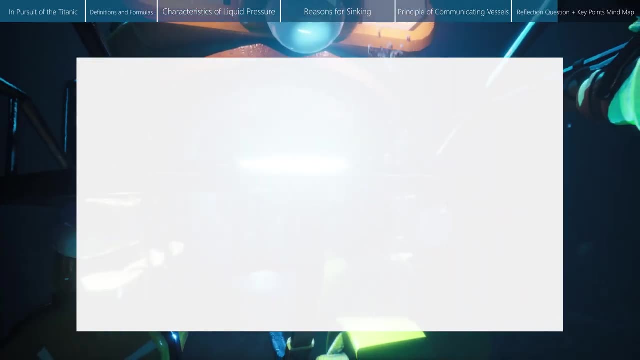 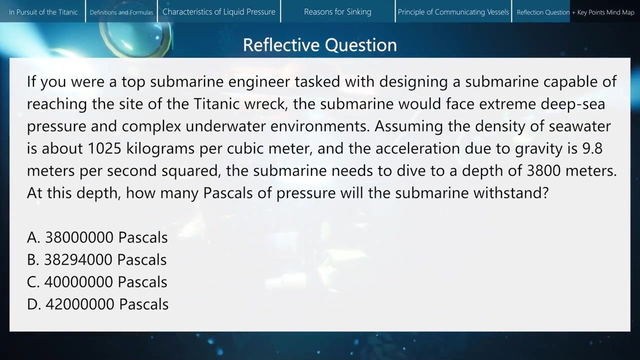 might trigger another, more severe accident, potentially causing failed damage to our submarine, leaving us forever in this unfathomably deep sea area. assume you are now the conductor of this steam train. our task is to move this massive train mounted cannon to a safe location. to accomplish this task, you need to calculate the work required to move the cannon and then decide how much coal.